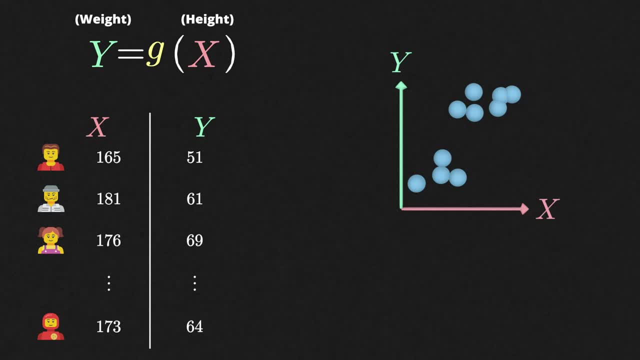 values for both x and y that we want to use to infer what the function g should be. We can then use that learned function g to predict the values y for new values of x not seen in training. Finding the right function g is called regression, and the easiest way to do this is to assume that this 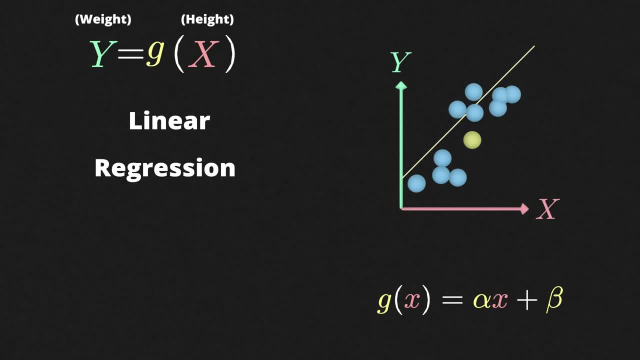 function g is a linear function, hence the name linear regression. Here alpha is the slope of this line and beta is the intercept. The simplicity of linear regression makes it really attractive. We're only dealing with linear functions here, so no complicated neural networks involved, If you. 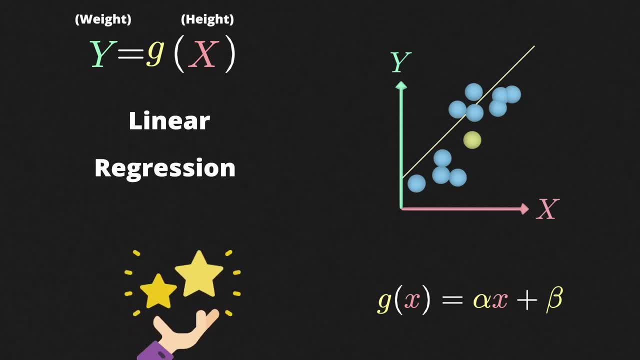 are faced with a prediction problem. linear regression should really be the first thing that you try To do. linear regression: we just need to pick the alpha and beta that makes this line fit the data as much as possible. One way to quantify the fit of a line to a bunch of data. 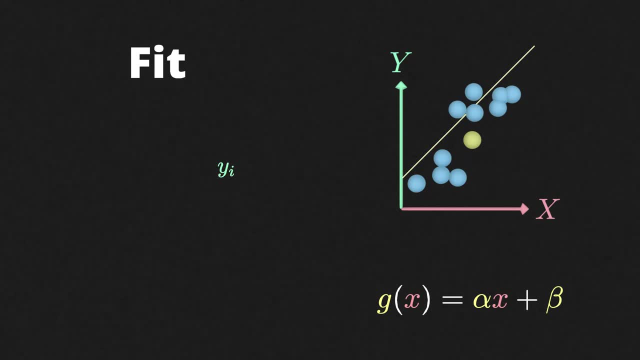 points is to consider where the point is, the training data set is and where it should be according to this line. take the square of the difference and then take the sum over all data points to find the alpha and beta that make this quantity as small as possible. let's take the gradient, set it to zero and solve for alpha and. 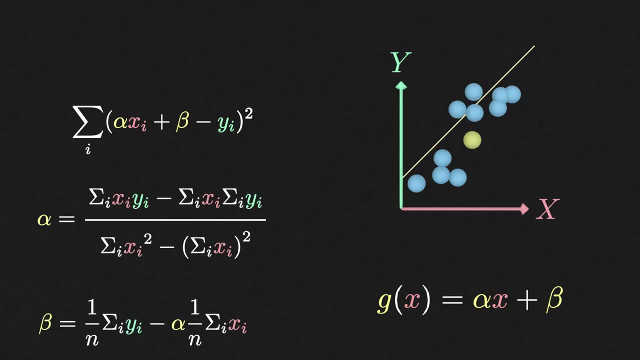 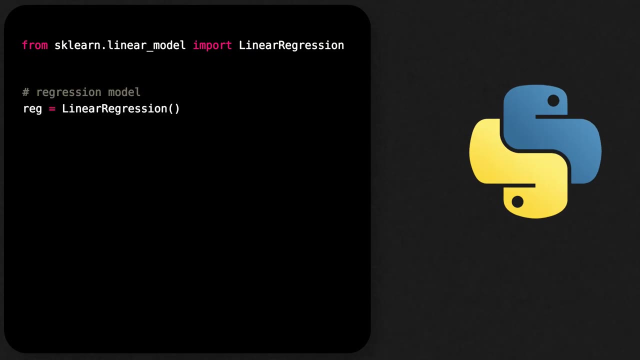 beta congratulations. you have just solved a prediction machine learning problem from scratch. if now you want to predict the weight of a new person, you just plug their height into this formula. in practice, you don't have to do this derivation by hand. if you feel more sophisticated, you can fire up python, import scikit-learn, declare a linear regression model and feed it the training. 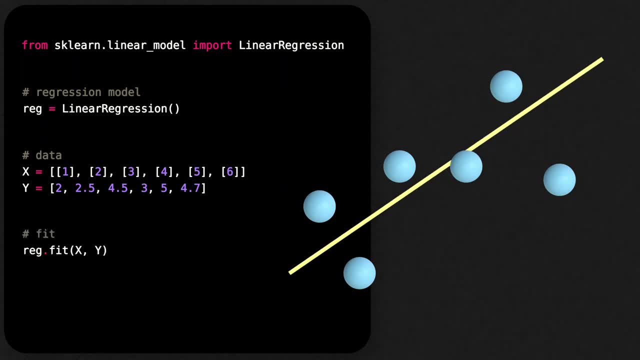 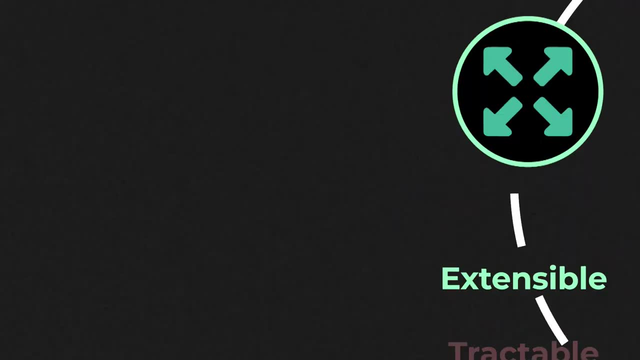 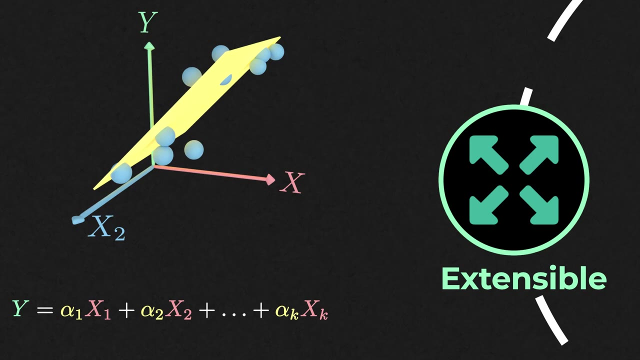 data and call the fit function to get predictions. you can just use the function predict. in addition to being simple and tractable, linear regression is also very extensible. for example, you can easily adapt linear regression to fit a model with more than just one variable as input. in the same vein, 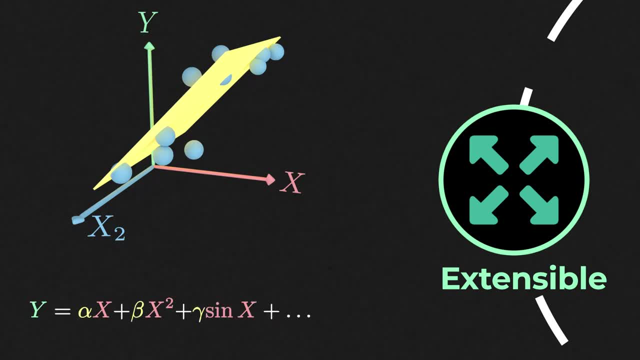 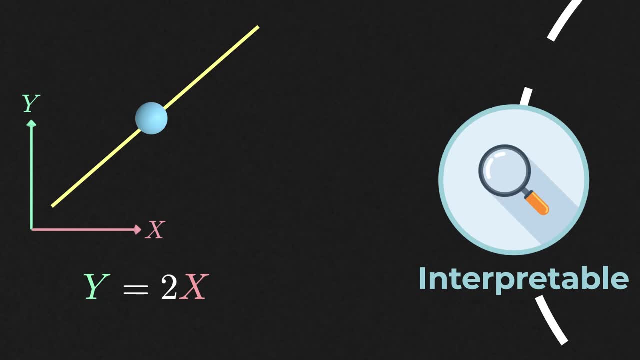 if you're not satisfied with a linear relationship, you can augment your data with non-linear features. another compelling aspect of the learning model is the ability to predict the weight of a line of linear regression, is the fact that we can interpret the coefficients that we get. for example, if the slope is positive, x and y move in the same direction, and if the slope is negative,